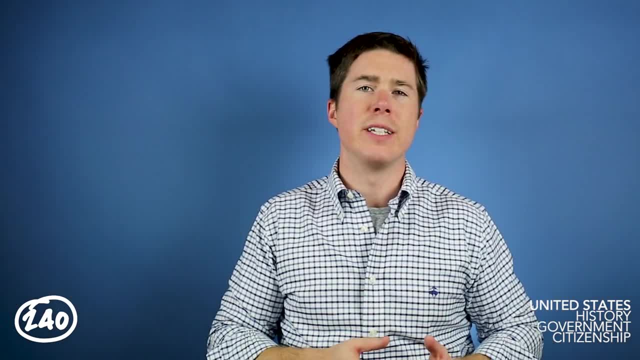 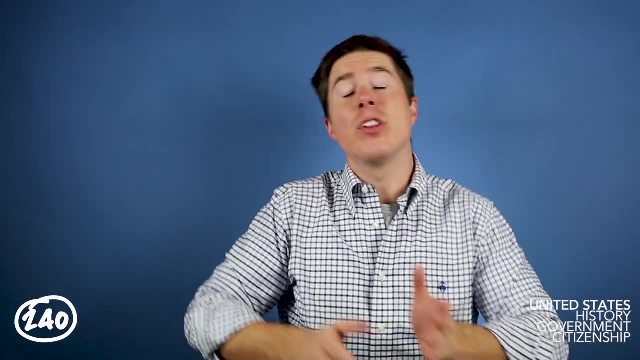 States. It's important to know the cause and effect of historical events. So as you study historical events, make sure you understand why the event is important and what effect that event had on the future of the country. Now let's talk about some of those major events and other. 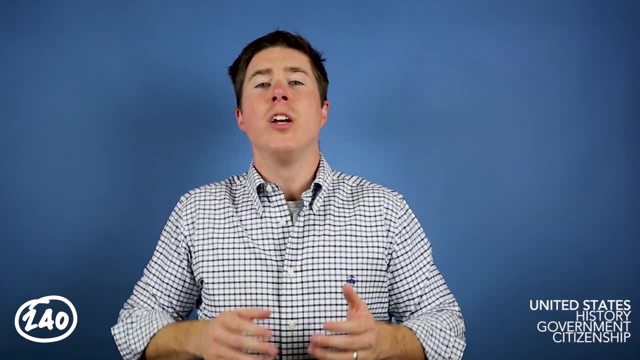 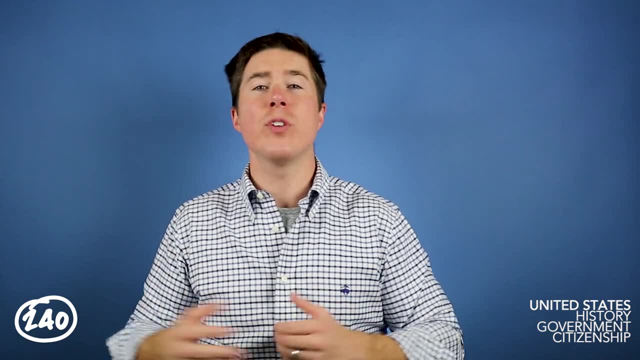 things you're going to have to know. The first is European exploration. You need to know why Spain, France and England explored the New World and colonized North America and what the results of those efforts were, Also know how Native Americans played into this. 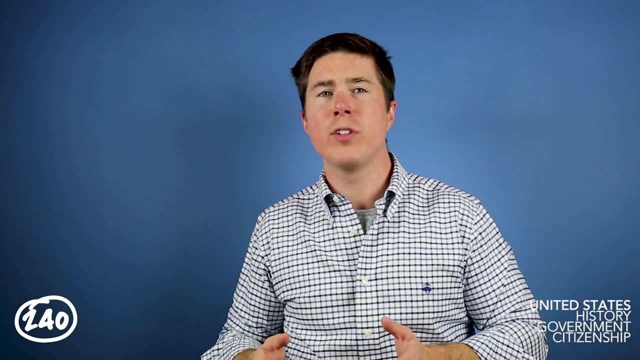 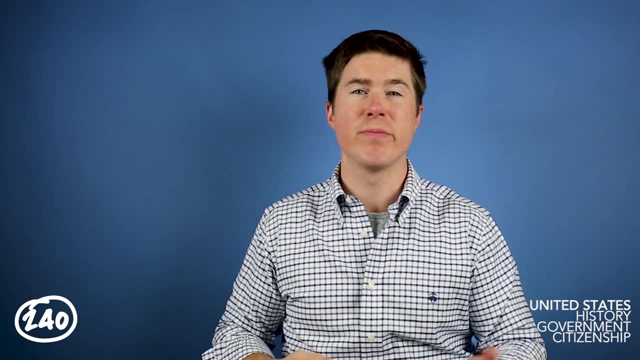 And the second is the American Revolution. Beware of the causes of the American Revolution, the key players and the key documents, like the Declaration of Independence, the Articles of Confederation and the Constitution. And, third, know major events and developments. These include things like slavery westward. 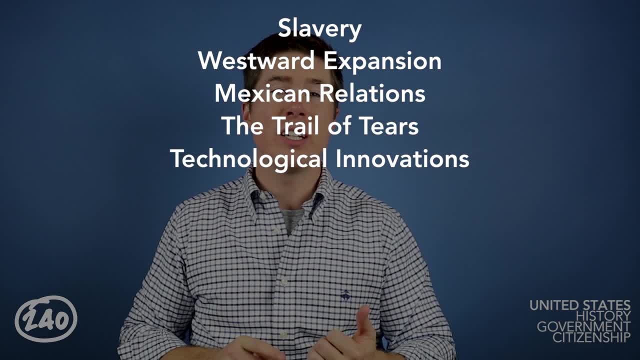 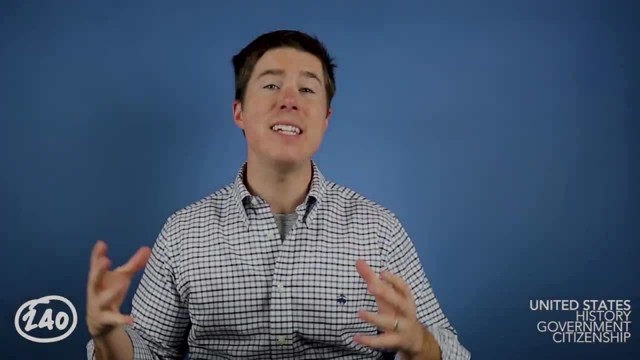 expansion, Mexican relations, the Trail of Tears, technological innovations, immigration, the Civil War, reconstruction, the industrial revolution, the progressive movement and women's rights. themes in United States history that you need to be familiar with. The fourth is 20th century developments. 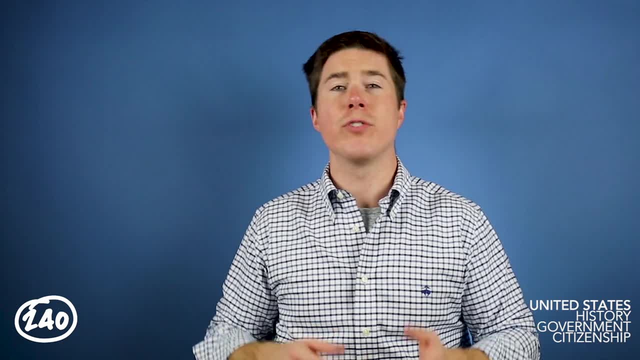 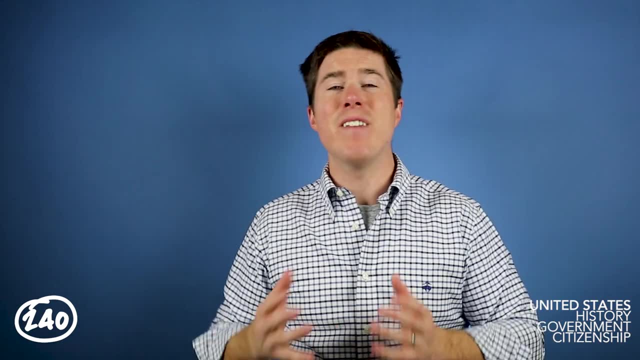 You need to know about America's role in World War I, women's suffrage, the Great Depression and the New Deal, as well as America's role in World War II, Vietnam, the Civil Rights Movement, environmentalism, changing demographics and the development of computers. 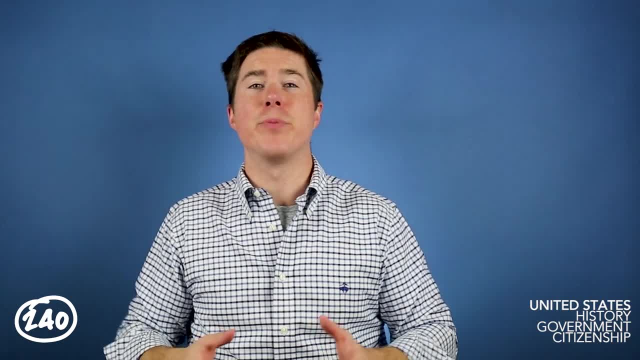 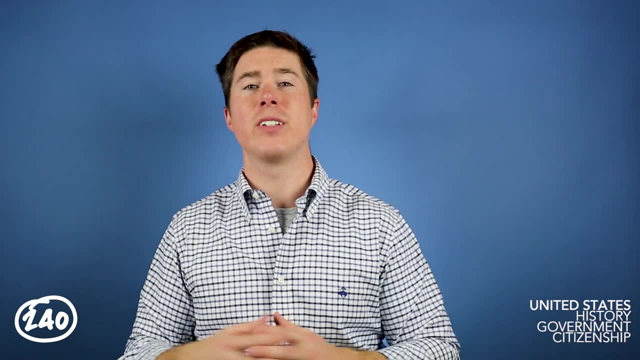 and information systems. And, finally, you need to be able to make connections between the causes of past events and their effect on future events. Now, this is a ton of information to have to study, and a really thorough study guide would be an excellent resource to have, and I know of a great one. but we'll get to. 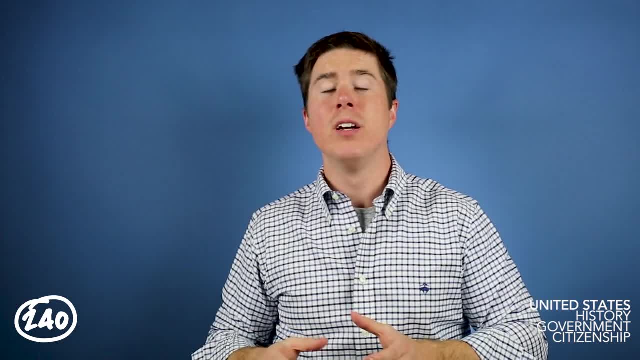 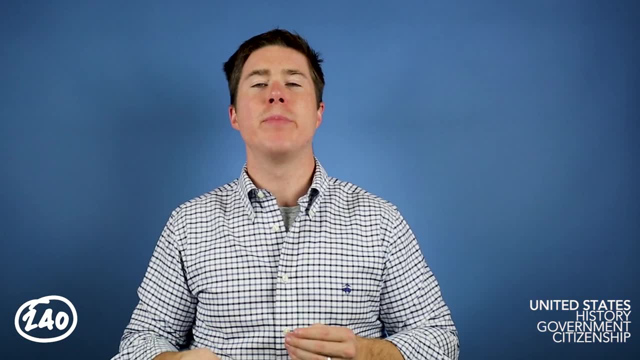 that later Now. the next big part is about government. This is the rules, the process and the people who make and enforce those rules and the processes. You need to know the purpose and responsibility and the relationship between local, state and federal governments. 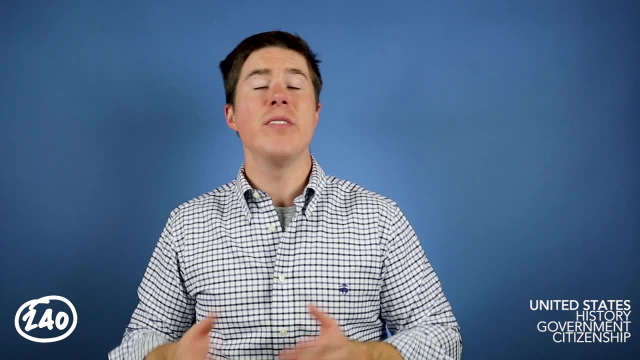 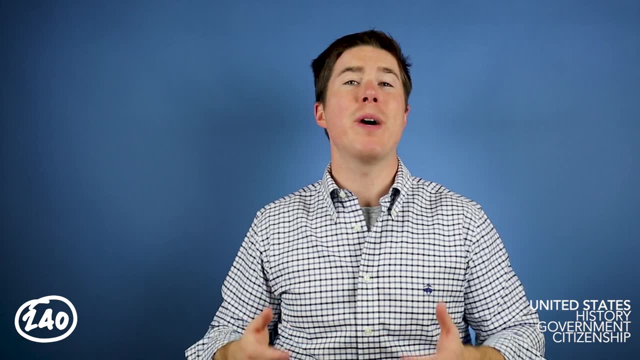 You also need to know the intended and unintended consequences of various forms of government, Be aware of the separation of powers among states. You need to be able to make connections between the three branches of the United States federal government, as well as the responsibilities of each branch. 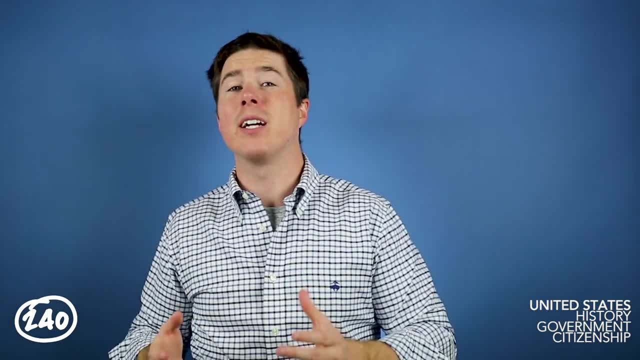 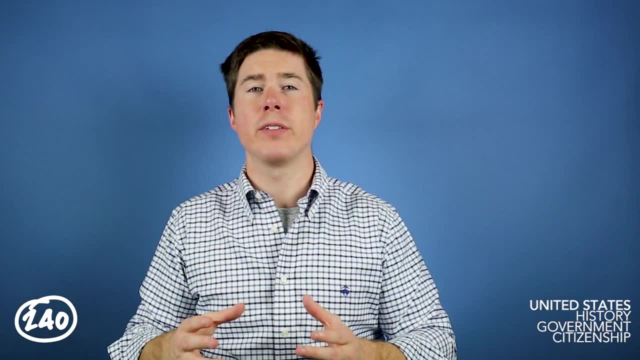 And finally know about the major documents and speeches in American history, like the Declaration of Independence, the Constitution, the Bill of Rights and the Gettysburg Address. These are impactful, important documents, And the last big topic is citizenship. 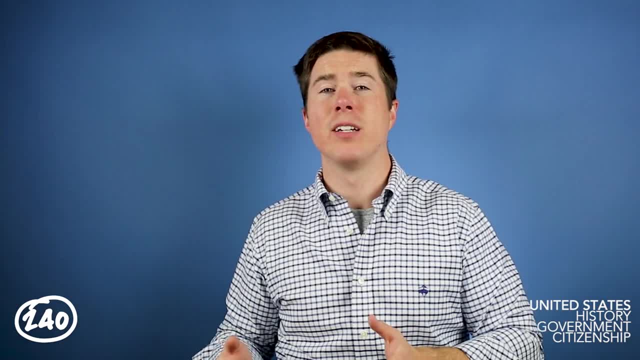 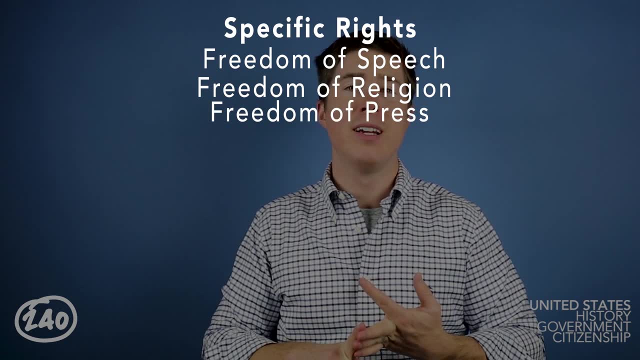 This includes knowing the rights and responsibilities of people in a democracy. Important topics to note and study include things like specific rights, freedom of speech, freedom of religion, freedom of press. We know these help in supporting government. now We know there are basic rights like citizen gef th madness and the roles that judge people. 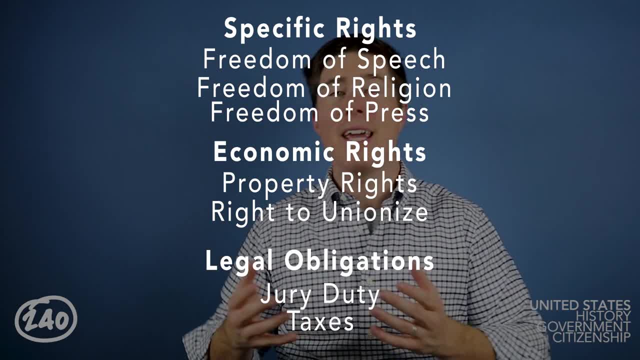 play. And then economic rights, Property rights, a right to unionize. They also include legal obligations of citizenship like jury duty and paying taxes. These included citizenshipft, starter duty. pension future got a lot in common. which examples of thoseights? 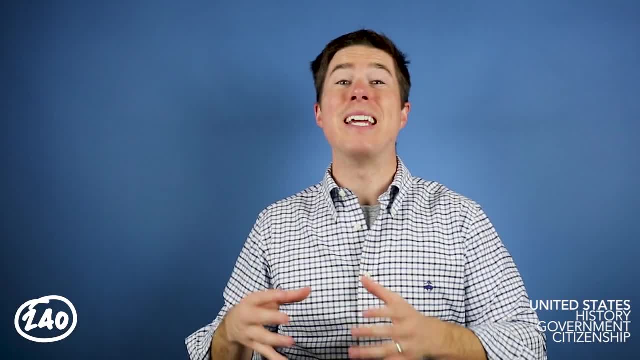 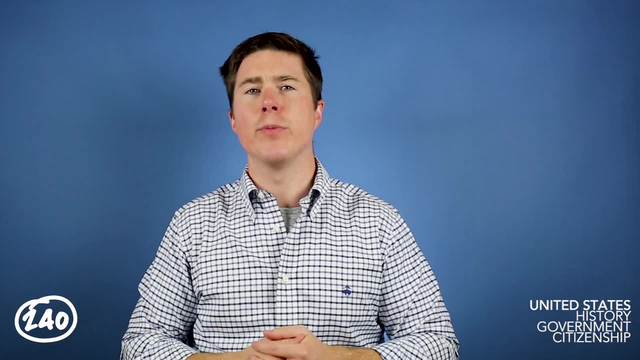 You need to know how all these work together to promote a common citizenship in the United States. Now, those are broadly the three parts to be familiar with concerning history, government and citizenship. so let's talk about three concepts with, in particular, the most likely. 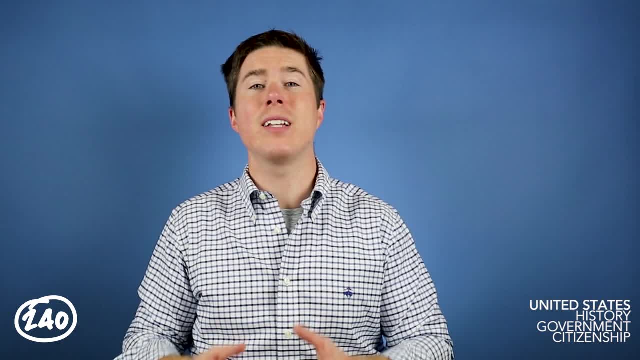 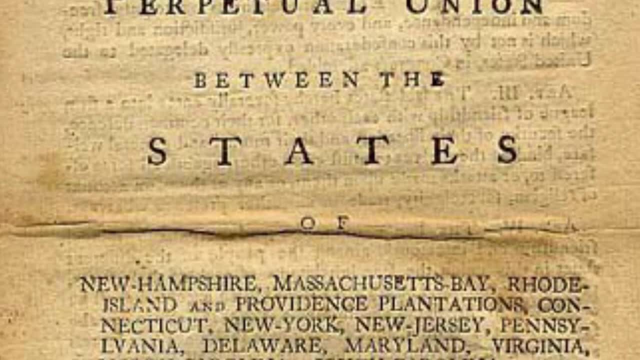 concept to be familiar with, since these will most likely appear on the test. This list includes area of the Constitution that would violate theoke högstens network 's items: The Articles of Confederation Or the Original Constitution of the United States of America. They're drafted in 1781.. They're a direct response to the complaints and the concerns. the colonies had with Great Britain. The article severely limited the power of the new national government and created a unicameral one-house legislature that required two-thirds votes to pass a law. It generally is considered a failure and replaced by the constitutional government of 1787, because so little got done and so little support of the federal government for the states. 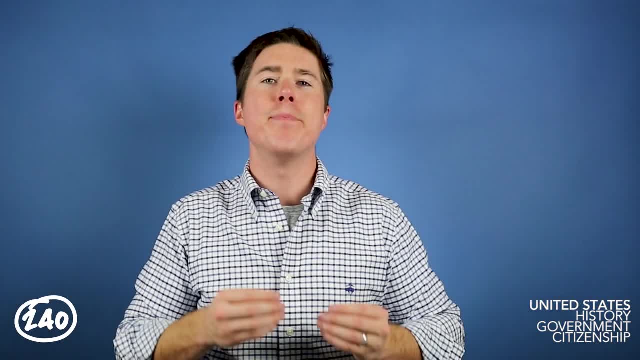 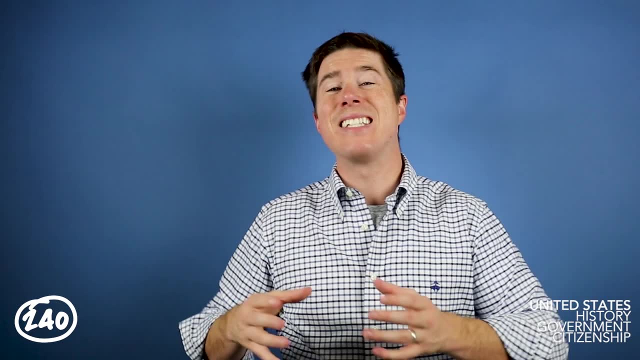 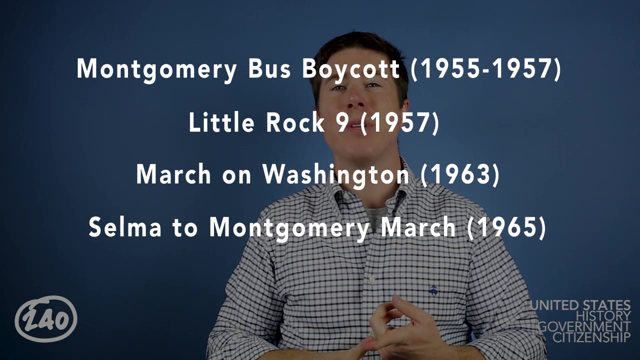 The next specific thing to know is the Civil Rights Movement, and this was a mass popular movement to secure equal rights for African Americans who faced racism and segregation. Some notable events in the Civil Rights Movement is the Montgomery Bus Boycott, the Little Rock Nine, the March on Washington and the Selma to Montgomery March. 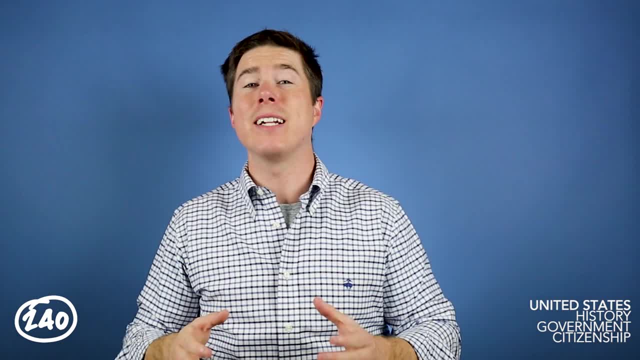 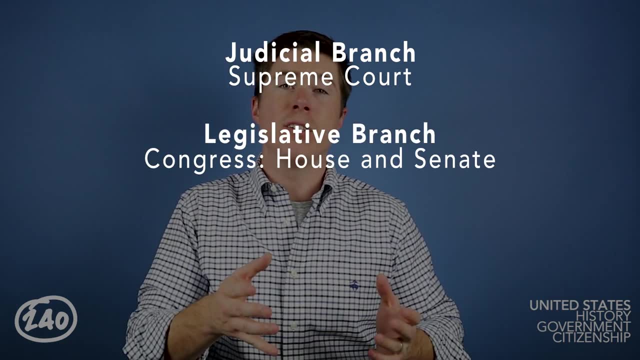 The next concept is that there are three major branches of the United States government. There's the judicial branch, headed by the Supreme Court. There's a legislative branch, which is Congress- It's the House and the Senate- Then there's the executive branch. This is the president. 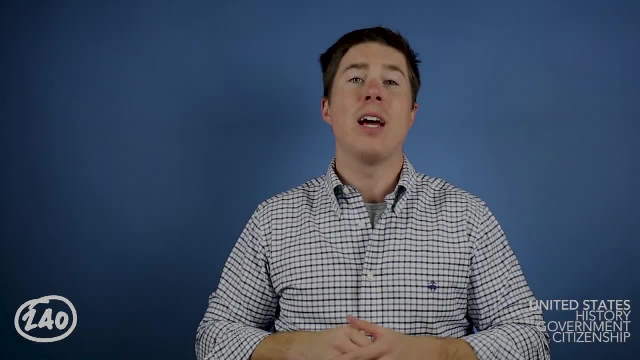 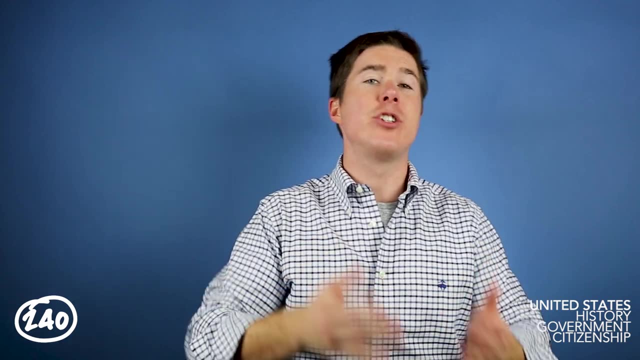 the vice president, the cabinet and generally the federal bureaucracy. Now you need to know how each branch works, who's in charge of what, and how the branches share powers and responsibilities, otherwise known as the checks and balances. Now, if all this seems, 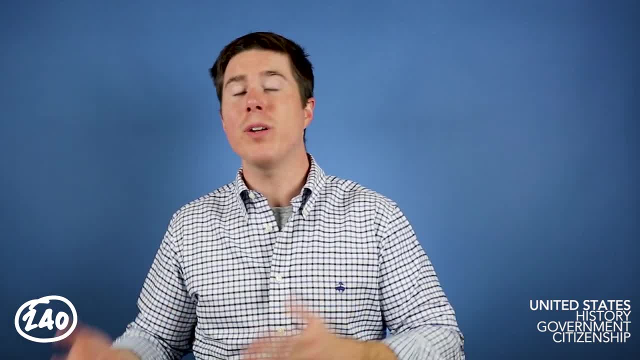 like a lot. it's because it is. There's a lot to know on the exam and if you want to pass it you have to study Now. the good news is- and I mentioned this earlier- 240 Tutoring has a great. 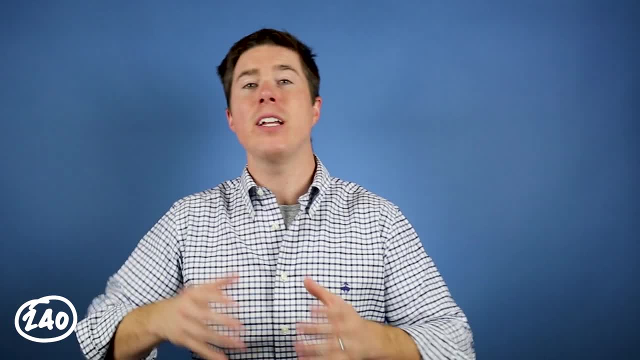 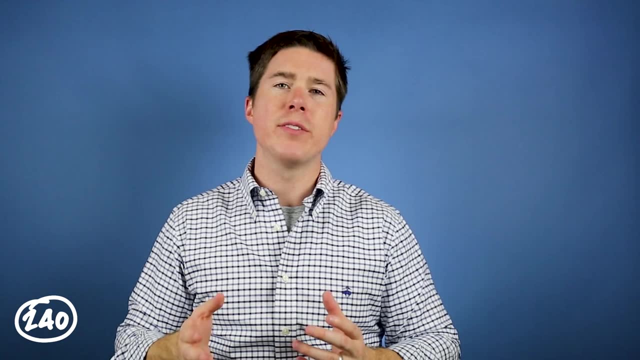 study guide, and we've done all the hard work of figuring out how to study, creating the best materials, creating authentic practice questions. Oh, and the test is also really expensive. so do yourself a favor: get something very easy, very simple to use and get a 240 Tutoring study. 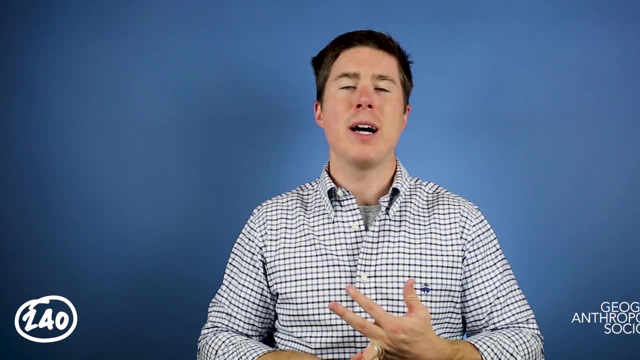 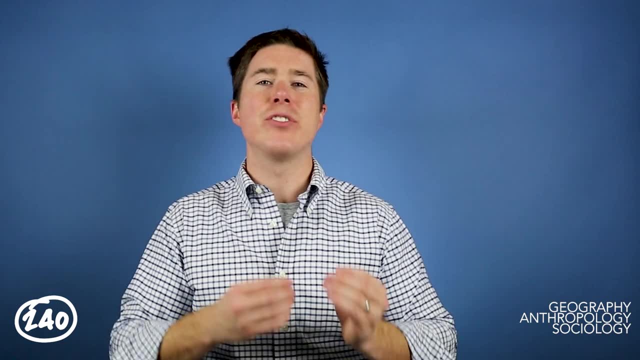 guide. Now let's move on to the next section: Geography, Anthropology and Sociology. This section tests your knowledge about the Earth and its people. Geography, Anthropology and Sociology questions make up about 30% of the social studies subtest. By looking at the exam's: 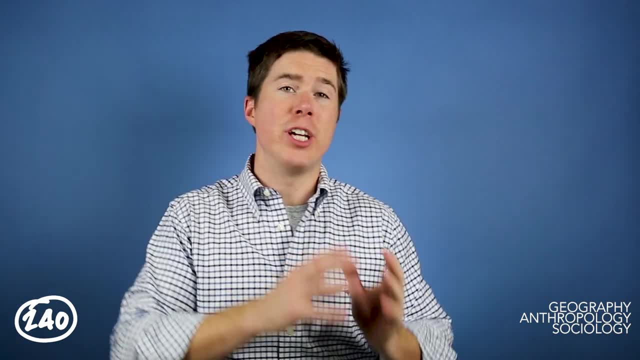 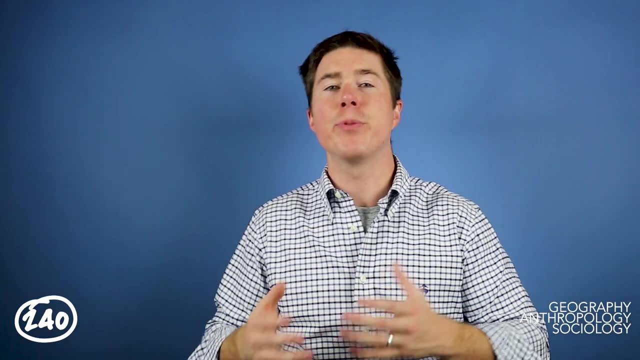 competencies. this section is already neatly divided into two parts: Geography, Anthropology and Sociology. Now, the first big part to know is Geography. Geography looks at the places and the relationship between people and those places. For these questions, you need to be able to read: 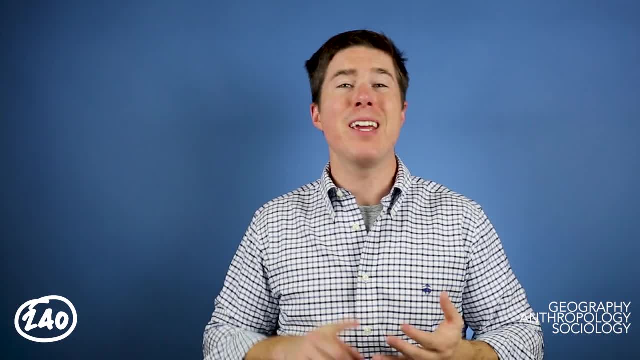 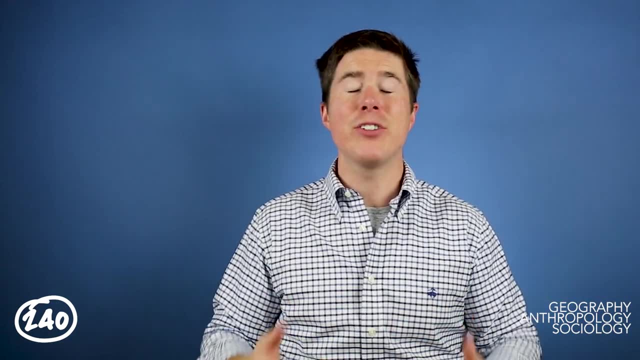 and interpret different kinds of maps, use the features of maps and be able to locate specific geographic features like the continents, oceans, major seas and rivers, major mountain races and major countries and cities. so know your way around a world map. Now you will see at least. 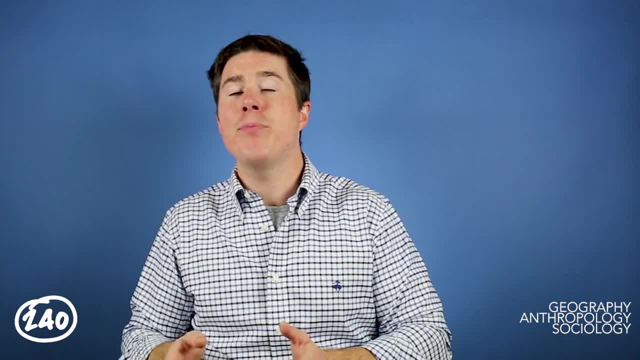 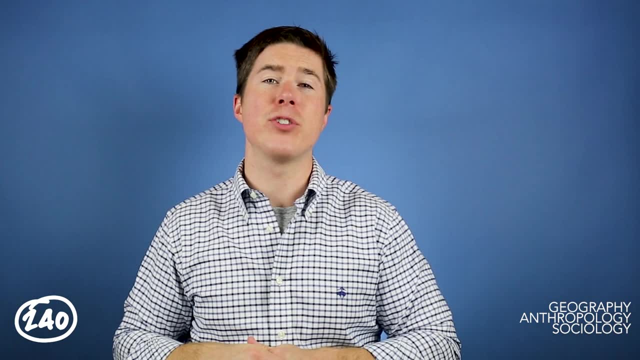 one map on the exam. You also need to know how the people and the environment are related to each other. This includes things like understanding seasons, weather, climate, settlement patterns, population trends, trade relationships, the effects of human on the environment and natural resources. 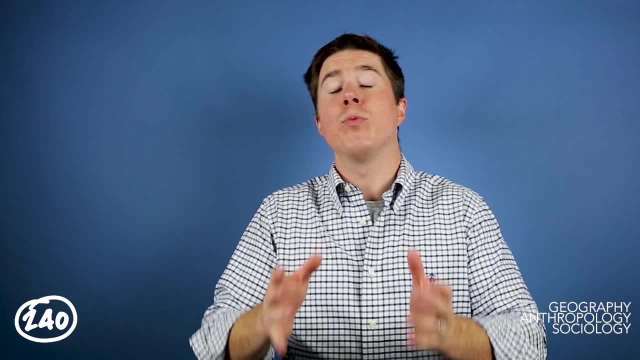 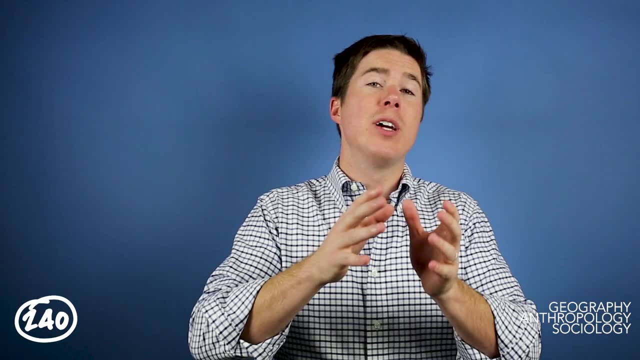 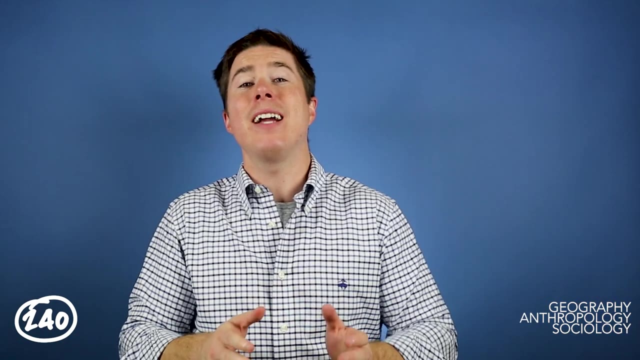 and ecosystems. That's a lot, But really all that means is how do humans respond to the environment that they're in? All those things I just listed is really a response in specific ways that people interact with their environment. Now, finally be prepared. 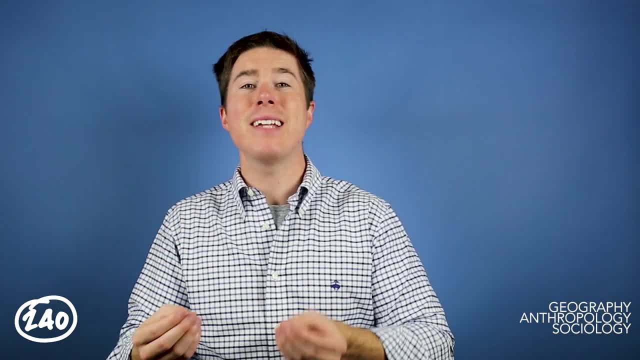 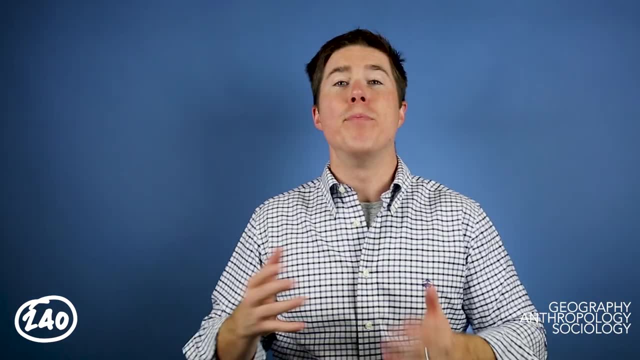 to answer questions about how we can use geography to help explain past, present events and plan for the future. The last big part to know is about Anthropology and Sociology. Both of these social sciences study people. However, the key difference is that Anthropology focuses on culture, while 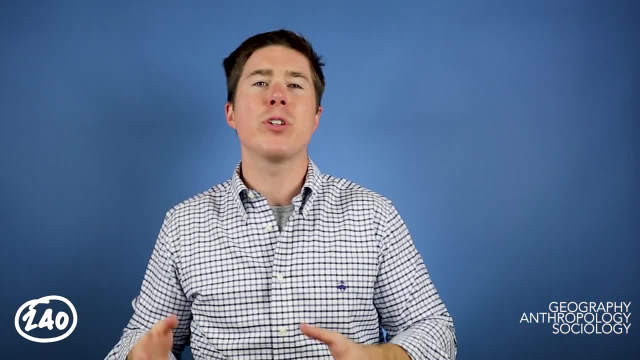 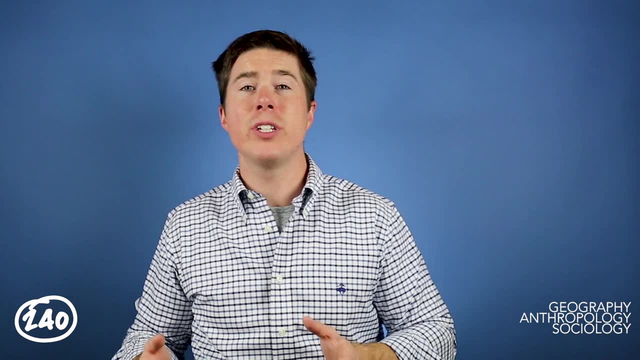 Sociology focuses on society. Now, when it comes to cultural geography, here's really what you need to study: How the family meets its basic human needs, the importance of social institutions, cultural expressions, social stratification and social relationships. How do cultural relationships, social communication and mobility, ethnic groups, general stereotypes. 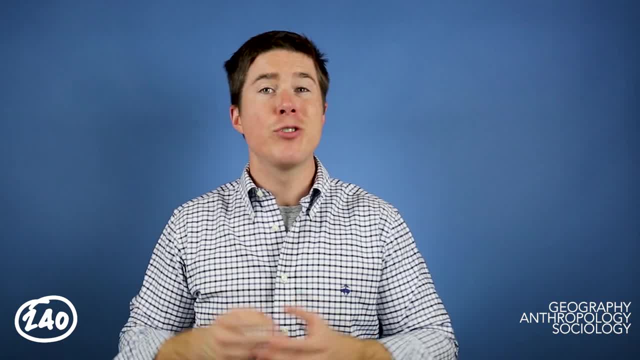 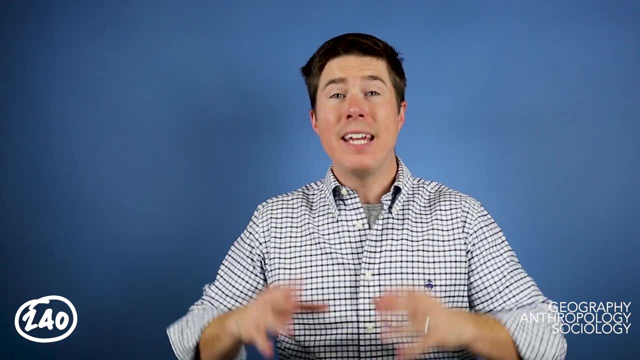 biases, values and ideals come about in a culture. Those are the two big parts to be familiar with Now. right now, I'm going to give you three specific concepts to be familiar with in this section, because they are almost guaranteed to come up on the test. 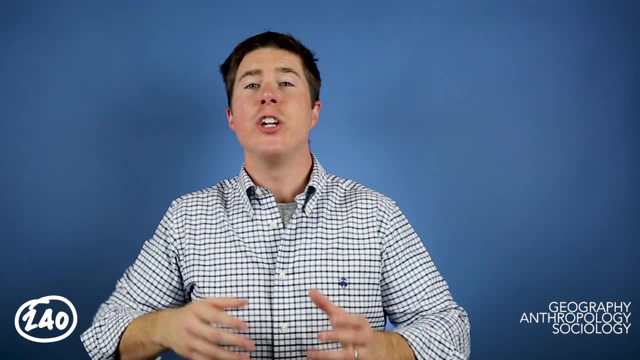 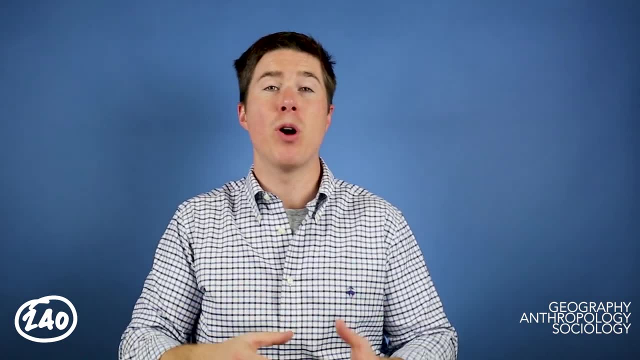 The first is maps, Because the earth can be hard to visualize. geographers use maps and globes to help them. Maps are two-dimensional renditions of a place. They can cover any area, ranging from a park to the whole world. The first is maps, Because the earth can be hard to visualize, geographers use maps and. globes to help them. Maps are two-dimensional renditions of a place. They can cover any area ranging from a park to the whole world. The second is maps. Because the earth can be hard to visualize, geographers use maps and globes to help them. Maps are two-dimensional renditions of a place. They can cover any area, ranging from a park to the whole world. 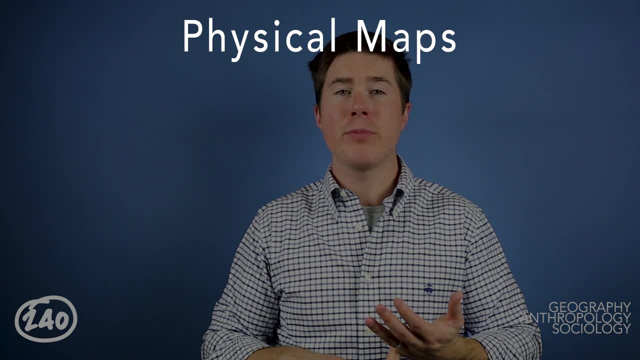 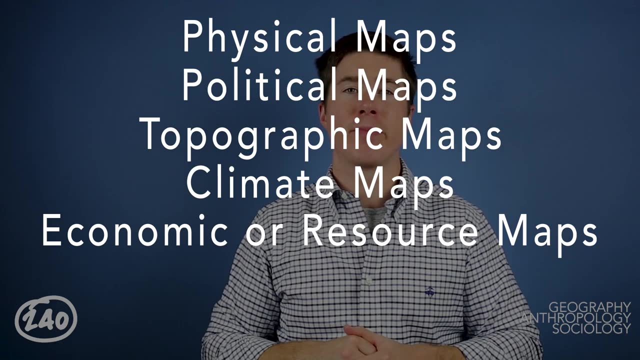 Now there are different maps that you will need to study, And they are physical maps, political maps, topographic maps, climate maps and economic and resource maps. Oh, don't forget thematic maps. You also need to know what features are on a map such. 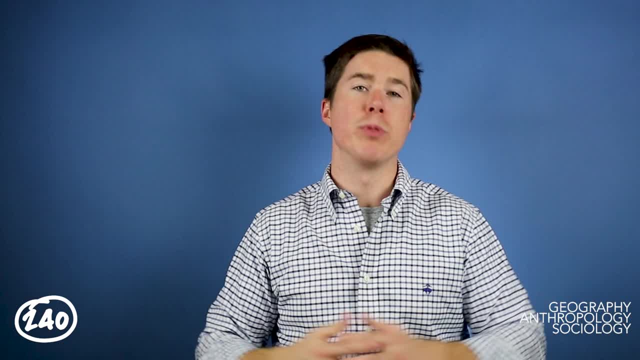 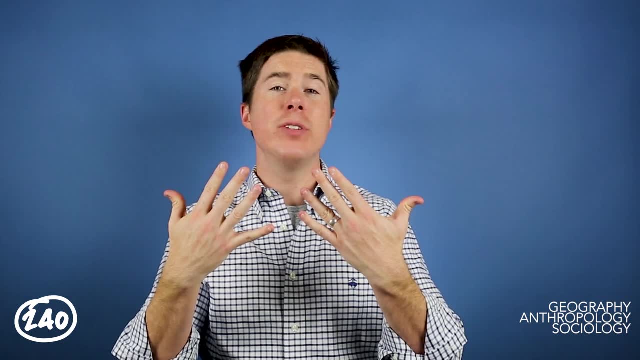 as a compass rose and a legend, and how to interpret it. Now. the second is climate. Climate is the average weather for a given place or location. There's ten distinct climates you need to know, And if you look in the description below, I will place a link for those climates and other great geography resources so you can specifically know what you have to study and learn the characteristics. So you're going to want to research each of these climates, provide examples of each and be able to differentiate them by their unique features. 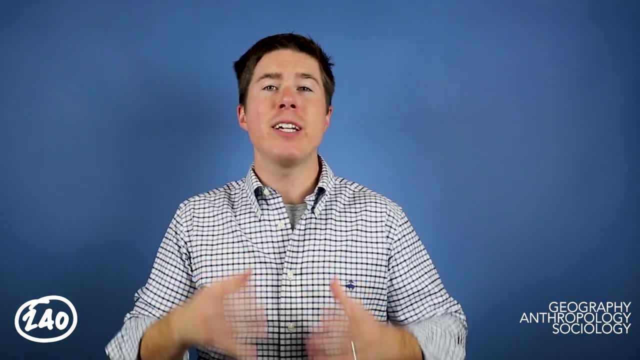 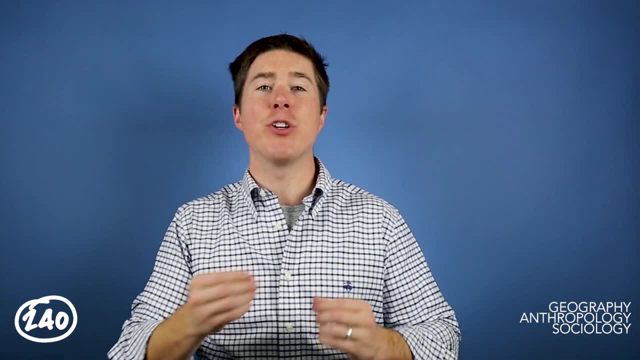 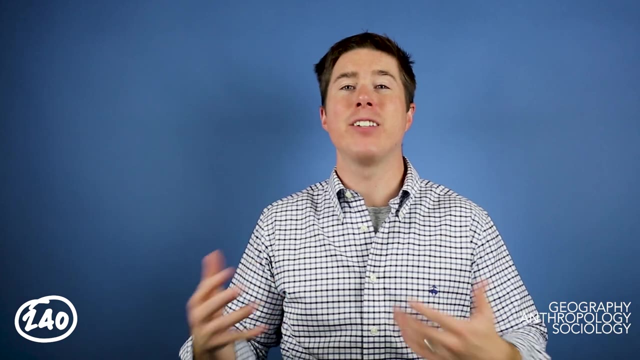 And the third: human-environment interaction. Geographers are particularly interested in the interaction between humans and their environment, specifically the way environment impacts the development of culture and how human activity shapes the environment. Human interaction with the environment resulted originally from efforts to obtain basic human 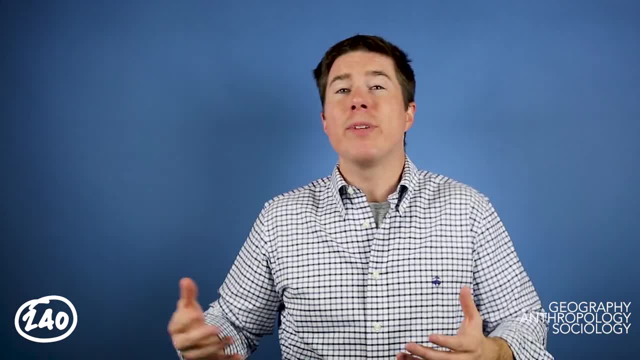 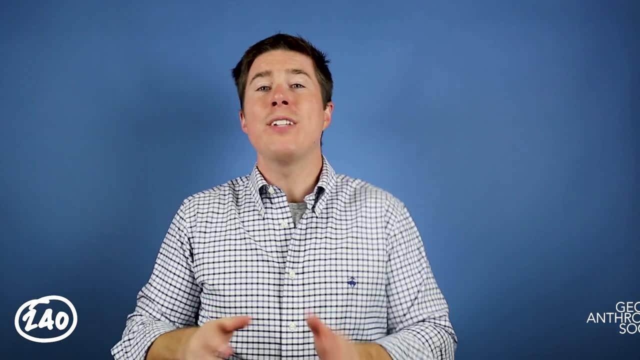 wants like food, shelter and clothing. Over time, as wants have become more complex, humans have exerted increasing control over their environment, attempting to shape it to their desires. So let's move on to the next section: world history and economics. Now this section tests. 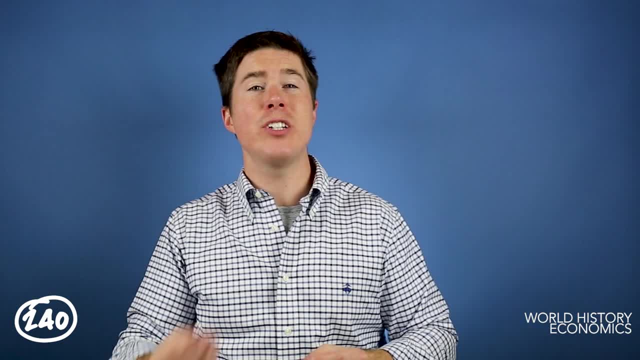 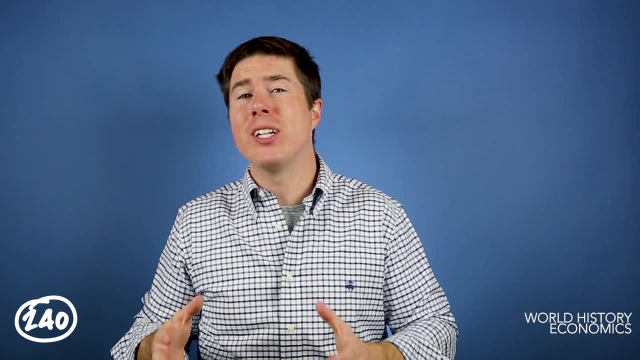 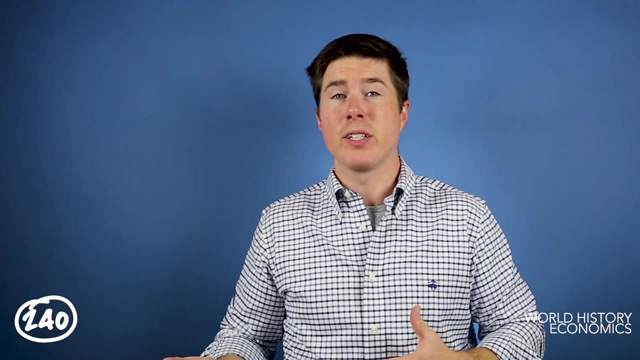 your knowledge about the major past events of the world and the production, distribution and consumption of goods and services, which is really economics. World history and economics questions make about 25% of the time. Now this section can be neatly divided into two parts: world history and economics. 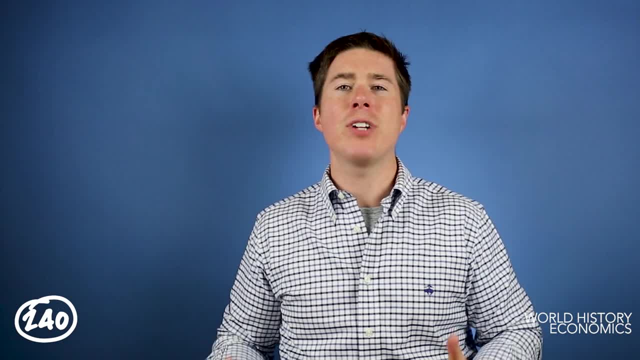 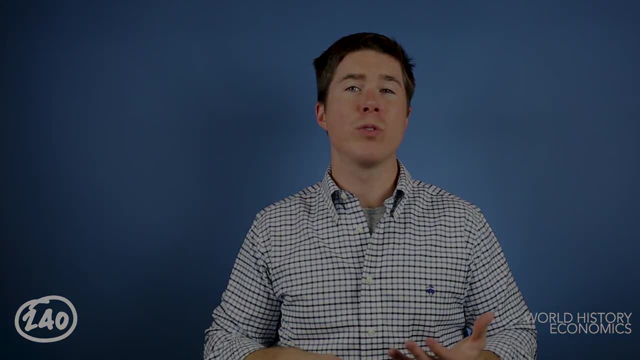 The first big part is about world history. You need to know the major contributions of Egyptian, Greek and Roman civilizations. Also know the major happenings of the 20th century, including World War I, the various worldwide revolutions, the worldwide economic. 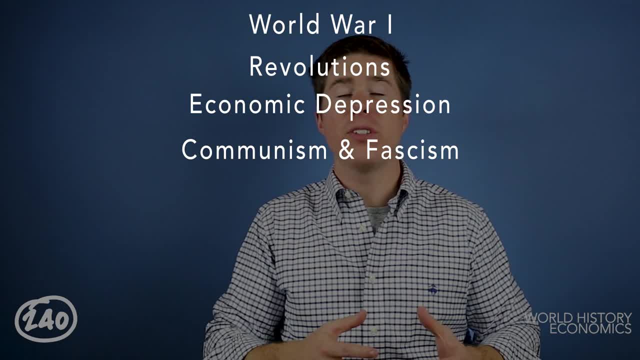 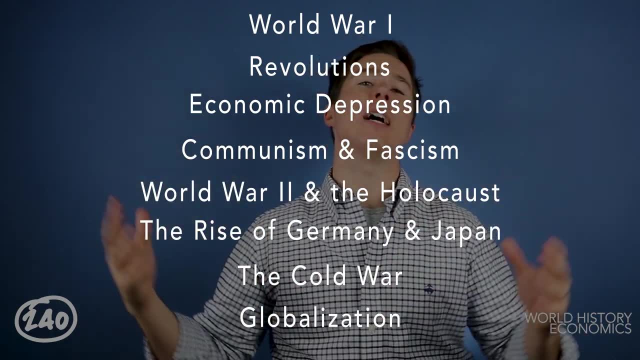 depression of the 30s, the rise of communism and fascism, World War II, the impact of the Holocaust, the rise of Germany and Japan, the Cold War, globalization. There's a lot to know, And the last big section studies economics. Simply put, economics is a study of production. 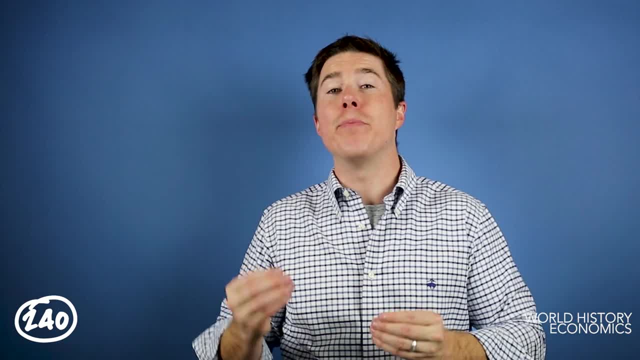 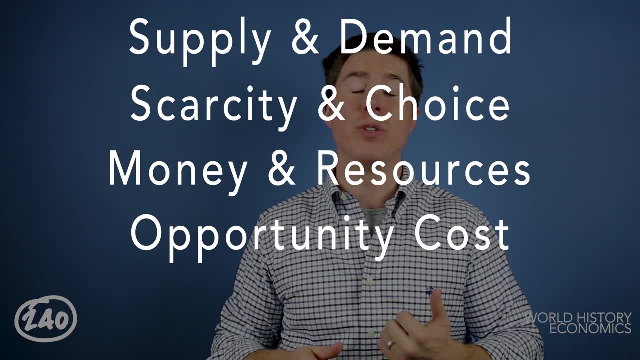 distribution and consumption of goods and services. So be sure to know the basic economic principles: supply and demand, scarcity and choice, money and resources and finally, opportunity costs. Also know the role of institutions like the Federal Reserve in how economics affects people. 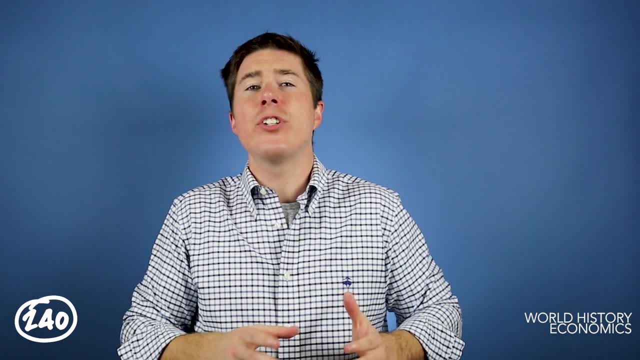 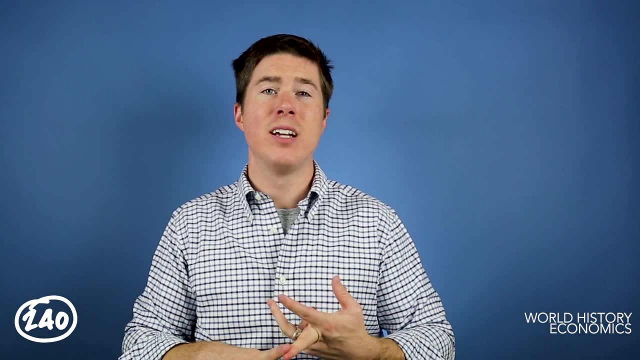 like the division of labor and specialization. Finally, understand what the role of government plays in economics. This includes understanding the purpose of taxes, currency, national debt, the consumer price index, how the federal budget works and, very importantly, gross domestic and gross. 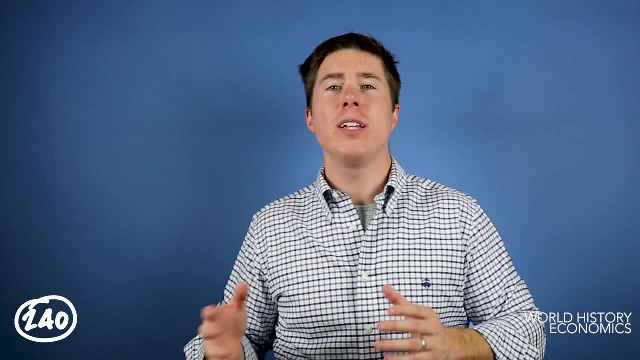 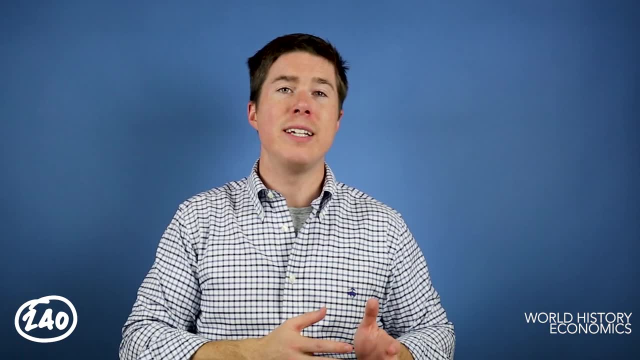 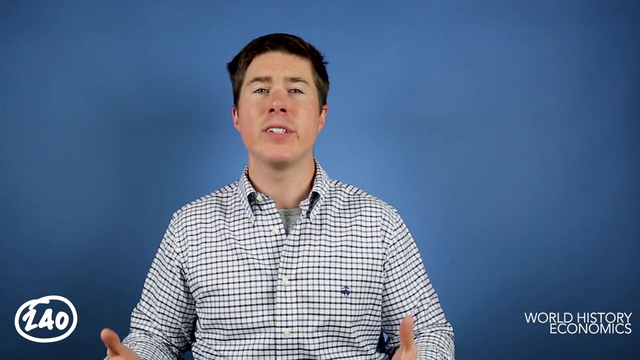 national product. Now, those are the big concepts to know. let's talk about three specific concepts. The first is going to be scarcity. Scarcity is the basic problem in the gap between our wants and needs and the available resources. No human has all the resources to fulfill all their wants and every need and every desire. 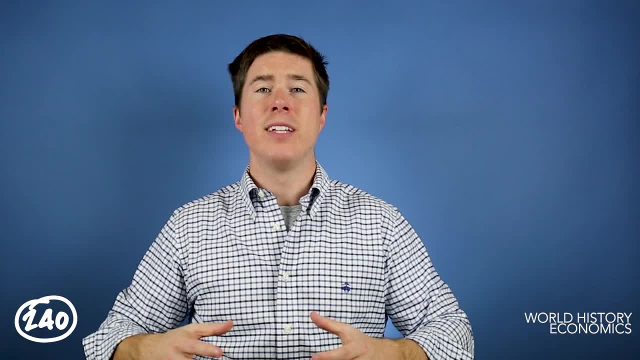 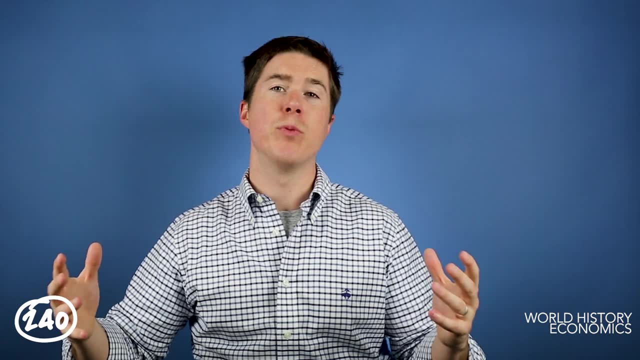 Because of this, people must use a cost-benefit analysis to make their choices. This means that they make trade-offs and decisions how best to allocate their resources, And if you're thinking that the richest man in the world has everything he wants, he's. 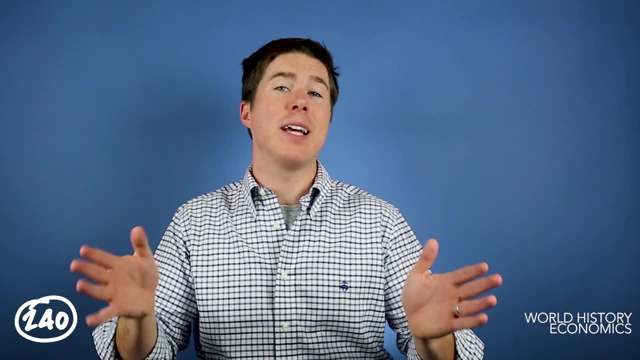 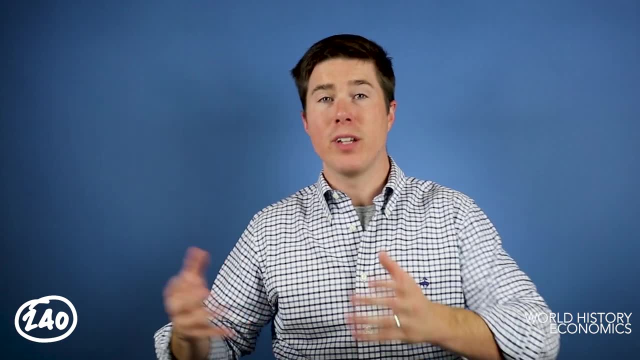 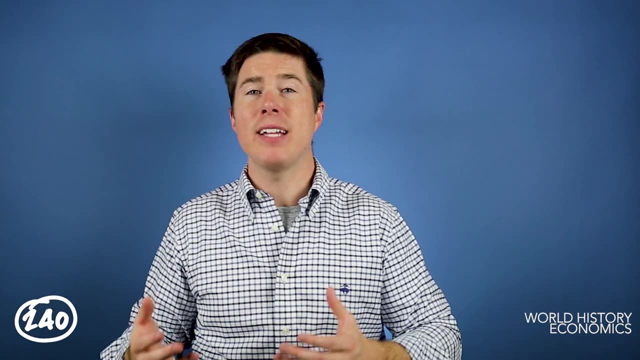 still constrained by time, So scarcity exists and applies to all people in the world. The second specific concept is supply and demand. In simple terms, supply is how much of something is made available and demand is how much the people want. There are a lot of factors that affect supply and demand and it's actually pretty complicated. 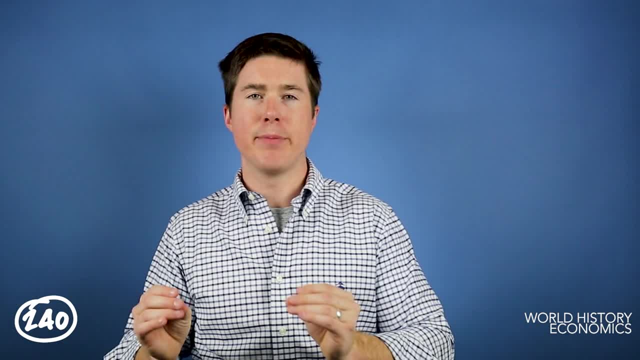 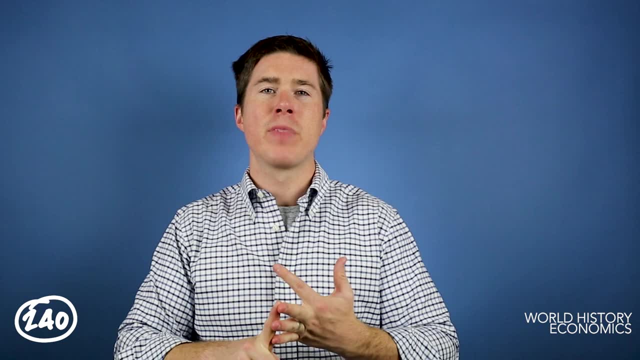 So take time to read about supply and demand and know the basic supply and demand graph. Now, if you're going to Google these things, look at the law of demand, the law of supply and the economics of scale When they become equilibrium and disequilibrium. look at what happens when you have a surplus. 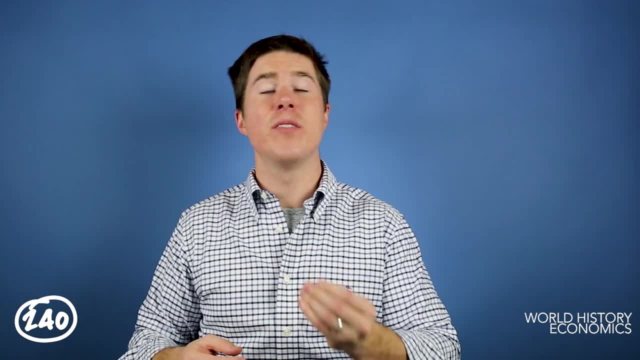 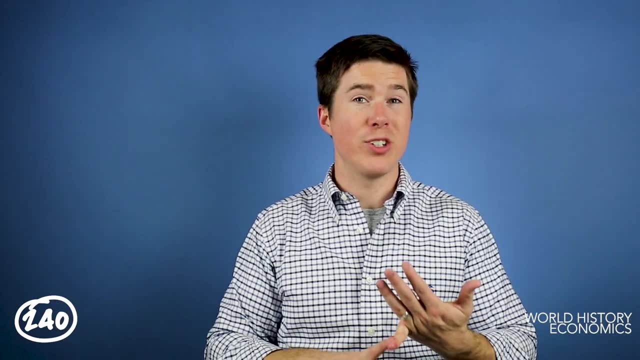 or a deficit and know the elasticity of those demand curves. Now, if you want to skip all that hard work, Just get a 240 tutoring study guide. It's got a great section on world history, all the events you need to know, plus on economics. 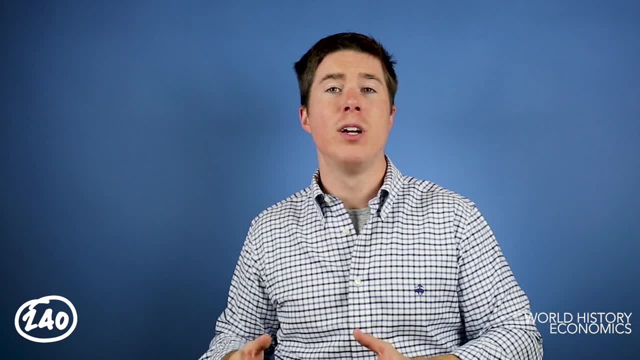 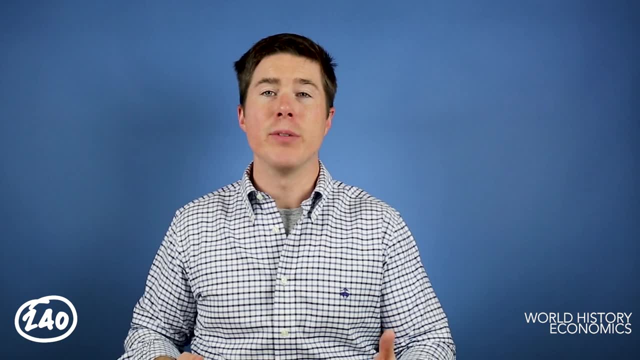 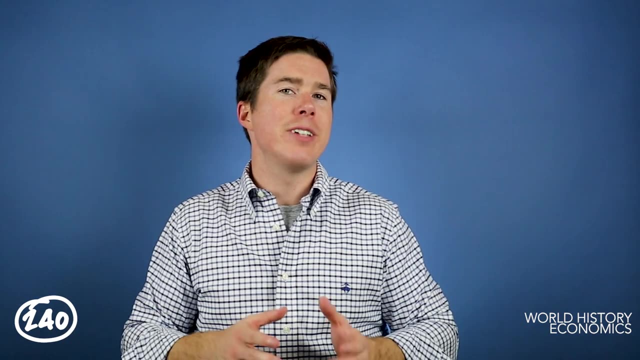 and it outlines exactly those big concepts that you have to know to get those questions correct. And, lastly, know the notable contributions from ancient civilizations, like ancient Egypt. You need to know their advancements in mathematics and the written language, like hieroglyphics in Egypt, and their agricultural technologies. 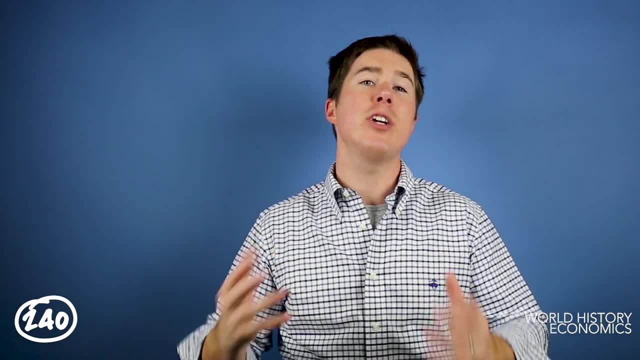 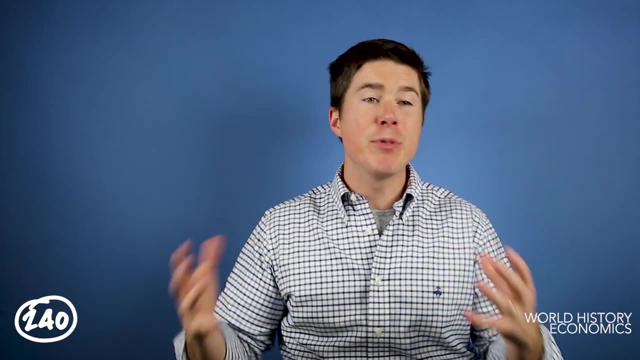 Now you also need to know the big achievements of Egypt, and there's none bigger than the creation of the great pyramids. These pyramids epitomize Egyptian cultural advances because they're geometrically perfect. The labor force was sustained through incredible agricultural advances. And lastly- and this helps with geography- they were insulated from attack from their neighbors because they were kind of surrounded by desert. So they were able to pursue these technological advances and create these monuments because they wouldn't have to worry about a threat of war from their neighbors. 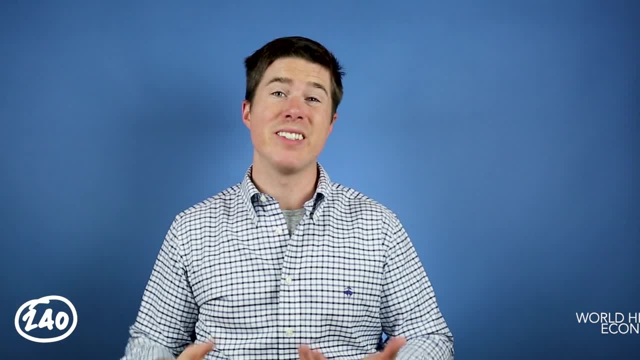 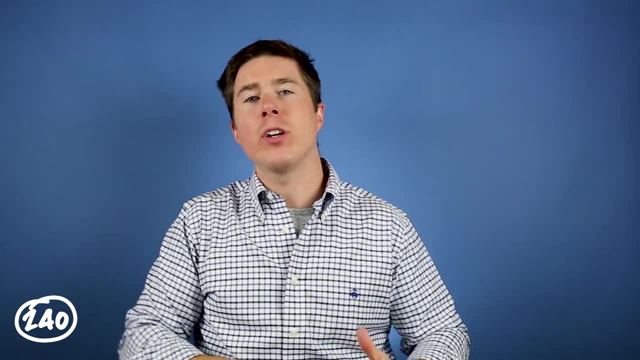 And lastly, if all this seems like a lot again, it's because it is. This is a huge test And it requires preparation. So if you have any question about what's on the test, what you need to study, where you, 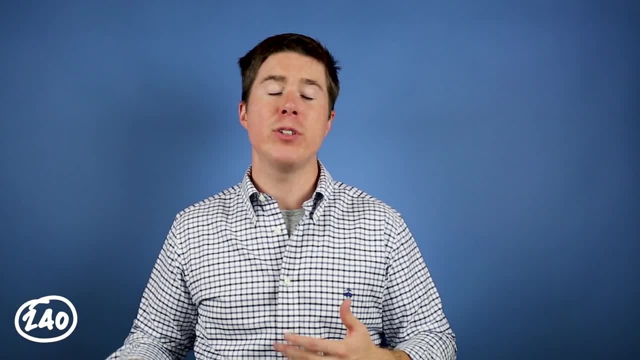 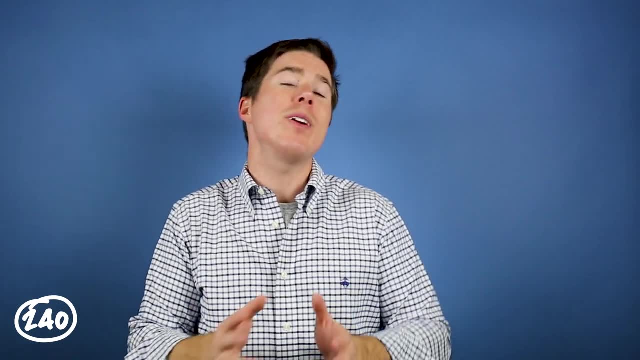 should start studying. just send us an email, admin at 240tutoringcom, Say I was watching your YouTube video and I have some questions. We're here to help you any way we can And we want to see you succeed on that test. 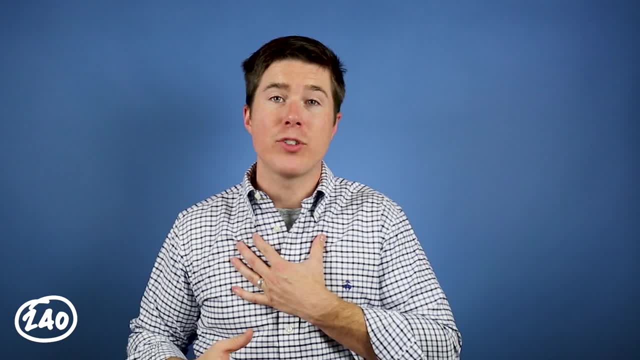 So go over to 240tutoringcom. you get to learn a little bit more about why I started the company- It's very personal- And you get to look at our study guides and see if they're right for you Now.